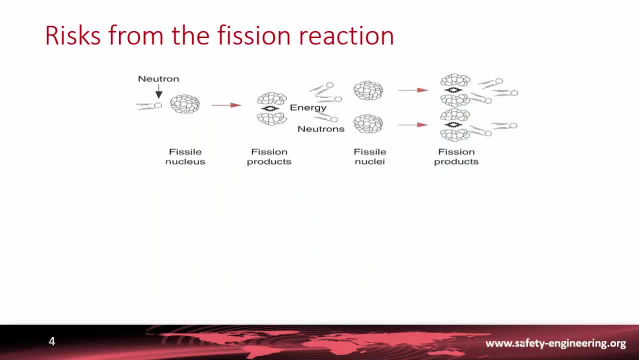 which is the major one. So what are the risks from the fission reaction? Of course, the immediate risk is that this reaction goes out of control. So there is the need to control the fission reaction. That's the immediate risk. but there is also a deferred risk, because even when the fission 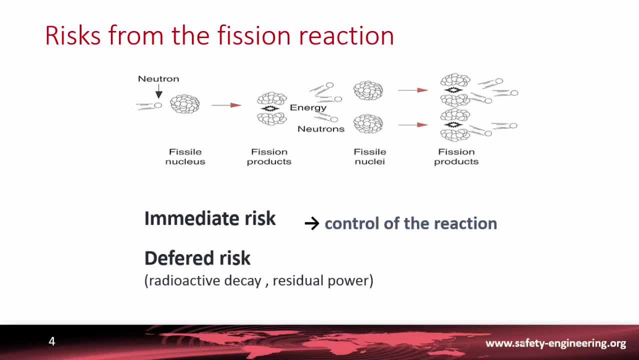 reaction has stopped. there is a lot of fission products which are radioactive. Even if they are decaying in terms of radioactivity, it remains what we call the residual power, and so there is a team: the need for long-term cooling after the shutdown of the reactor. 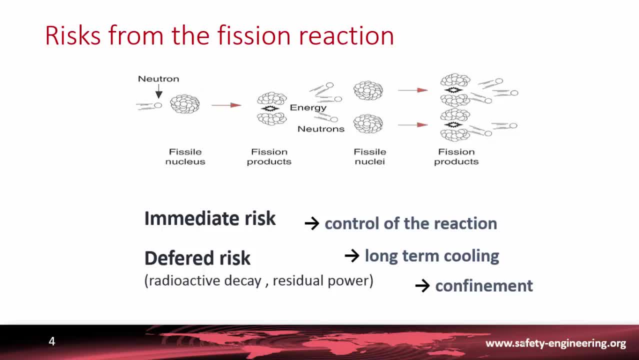 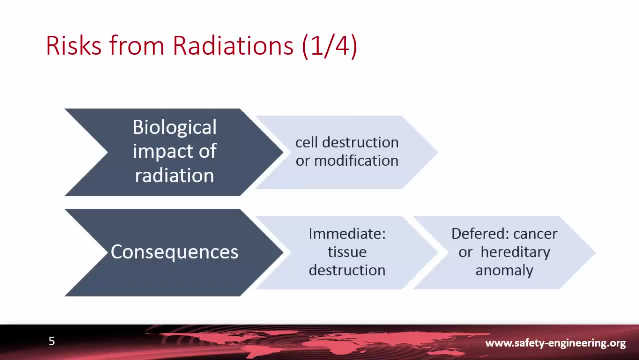 And another element very important to control is the confinement in order to avoid the radioactive products to escape. So let's talk about the risk from radiation. We have to know the risk of radiation in order to survive and get to the environment. So now the the risk from radiation. Radiation has some biological impact on the cells. 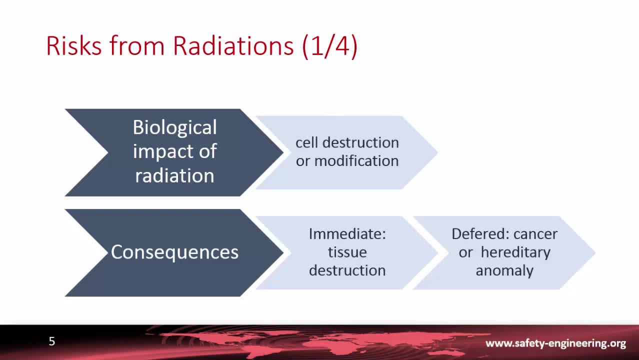 either destroying them or modifying their structure. So there are two kinds of consequences of that tissue: that it's like exactly like what when you got a burn. but there is also a defer effect and the, the modification of cell could lead to some cancer or to. 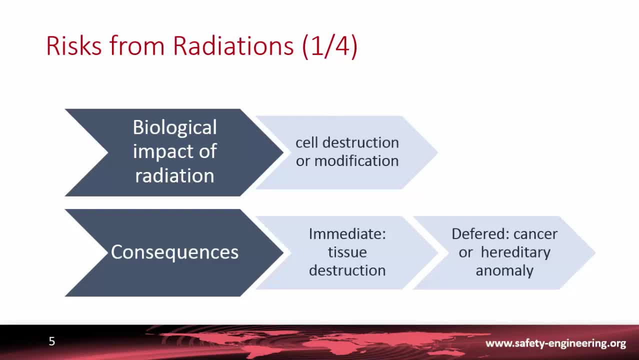 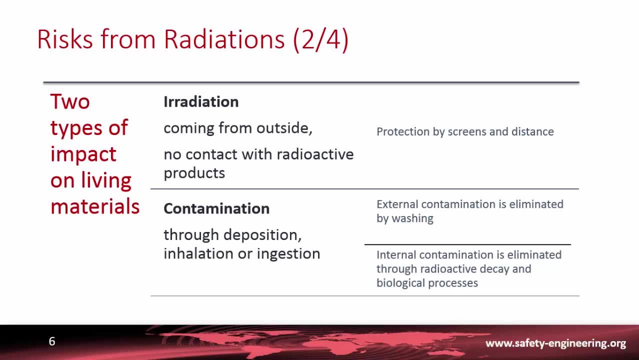 some hereditary and anomalies. there are two ways of impacting living material from radiation. we call the first one irradiation. it's a situation where the radiation comes from the outside and this would occur without any contact with radioactive products. the way to be protected against irradiation is by 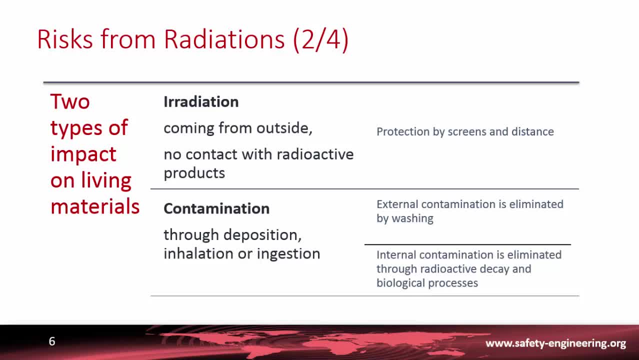 putting some screens or increasing the distancing between the source and the the living material. Another way of being impacted by the radiation is through what we call contamination. This happens when you ingest some contaminating products or inhale press ring or if you are touching some deposit of radioactive products. So if the contamination is outside this, 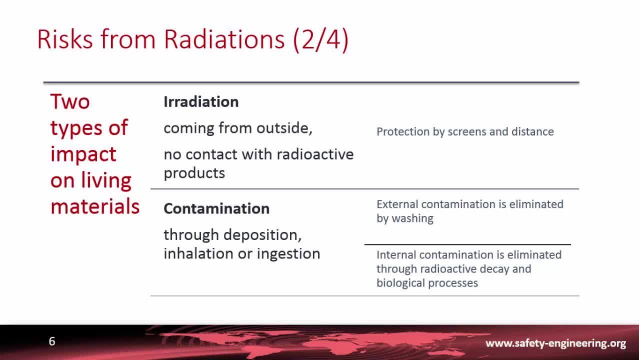 could be eliminated by washing, and this is a reason why each time you exit the nuclear plant, you have to wash your hands, and if you are contaminated you have to go through a shower. And if you happen to inhale or to ingest some contaminated products, 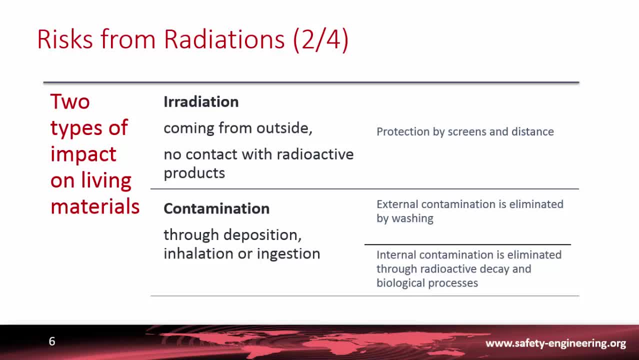 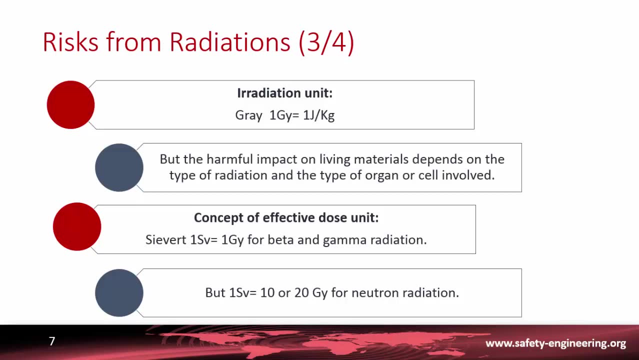 the elimination is done through the decay of the radioactivity or through biological processes. So the unit used for measuring the impact of radiation is the gray, and the gray is equivalent to one joule per kilo. But the harmful impact on living materials depend on the type of radiation. 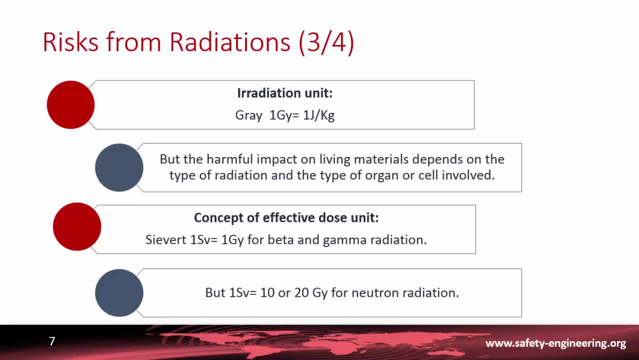 and the type of organ or cell involved, and it's not the same for a neutron or a battery, And so we use this concept of effective dose unit and it's the most used, and if you hear the the media, you hear talking about sieverts or 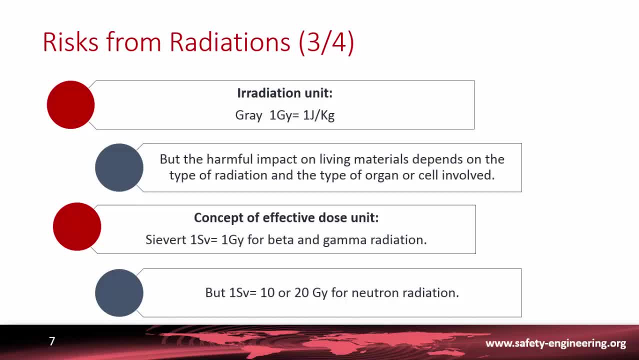 millisieverts, So One sievert is equal to one gray for beta and gamma radiation. but the impact could be much more important for the neutron radiation, and in this case one sievert is equal to 10 or 20 grays. 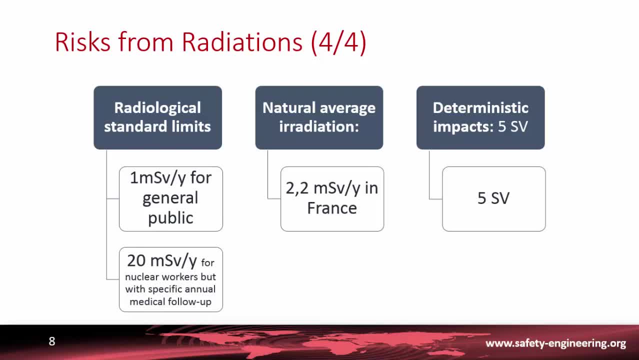 There are strict limits for radiation through regulation and standards. For the general public, the annual dose is 1 mSv per year, but for nuclear workers who have specific annual medical follow-up, the maximum allowed dose is 20 mSv per year. 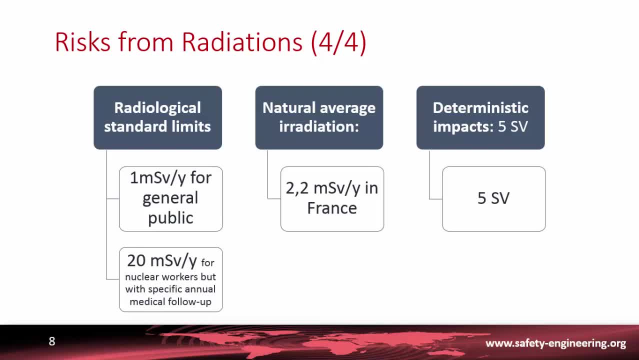 We have to compare that to natural average irradiation which for instance in France is 2.2 mSv. But in some other parts of the world, for instance in some part of India, the natural average irradiation could reach 10 mSv per year. 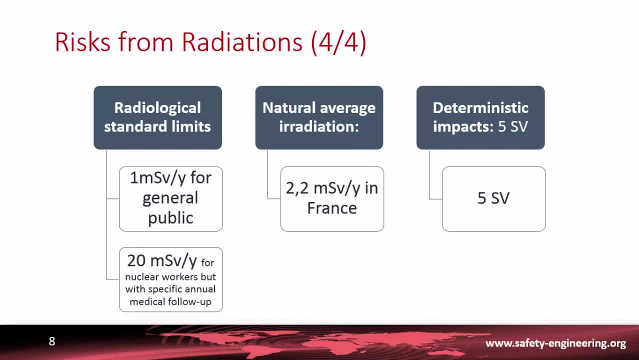 And the impact on radiation depends also on the quantity of radiation. The figure of 5 sieverts is something important because this is the beginning of the point. when you have some deterministic impacts, That means that it's certain and there is a proof that this kind of dose has a specific impact. 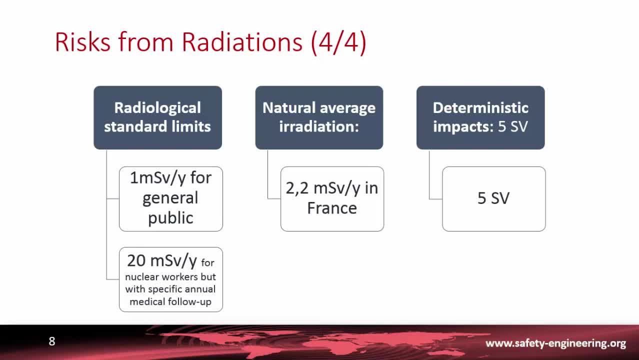 Below this value of 5 sieverts, we talk about stochastic effects. That means that for this low dose, you have a specific impact. Below this value of 5 sieverts, we talk about stochastic effects. That means that for this low dose, you have a specific impact. 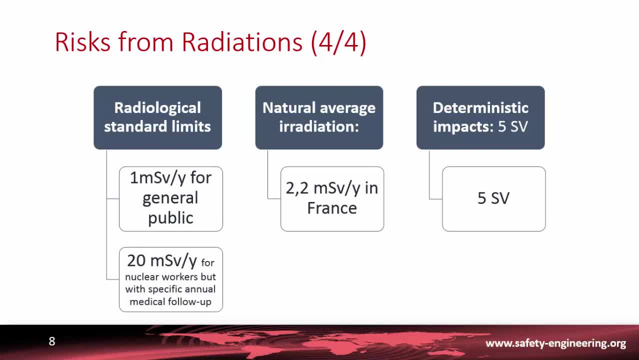 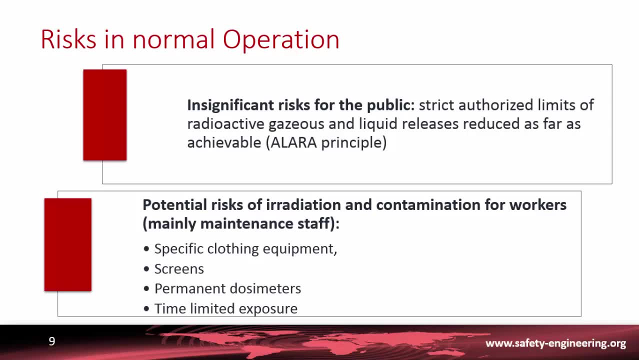 So you have to have a certain probability of having an impact, but it's not something certain. So you have to have a specific probability of having an impact, but it's not something certain. So you have to have a specific probability of having an impact, but it's not something certain. 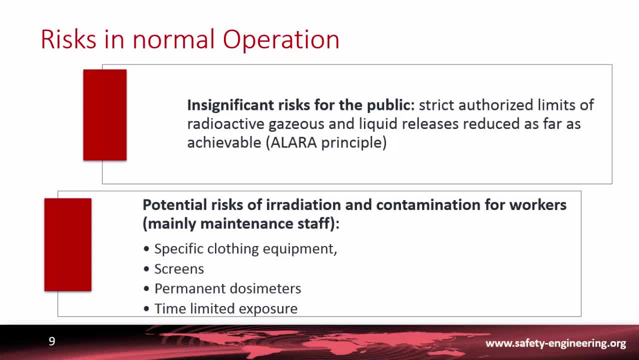 Let's now have a look at the risk in normal operation. First to say that for the public, in normal operation, the risk is completely insignificant Because of a strict authorized limit of both radioactive gaseous and liquid releases. And there is this principle of halara, which means as low as reasonably achievable. 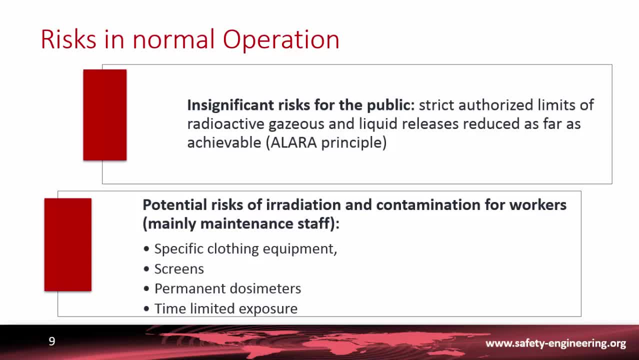 and this is a principle which is applied on all nuclear facilities- where, if there is something that could reduce the release in either form, the measure that should be taken to implement these elements and reduce again the dose incurred by the public, For the workers and specifically for the maintenance staff. 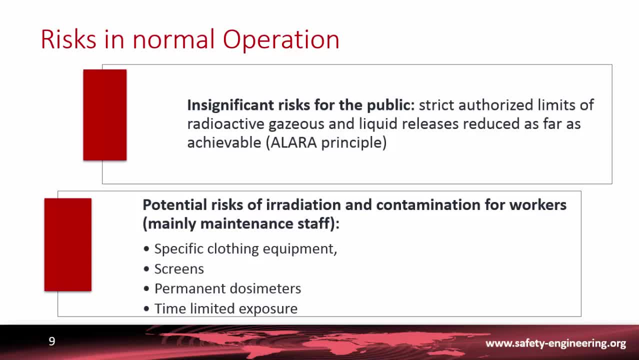 there is some risk of irradiation and contamination because of course they were closer to the source of radiation. So the measures which are taken to reduce this risk is wearing of specific clothing equipment, including some scaphandria. We use also LED screens around the piping when there is some contamination inside the pipe. 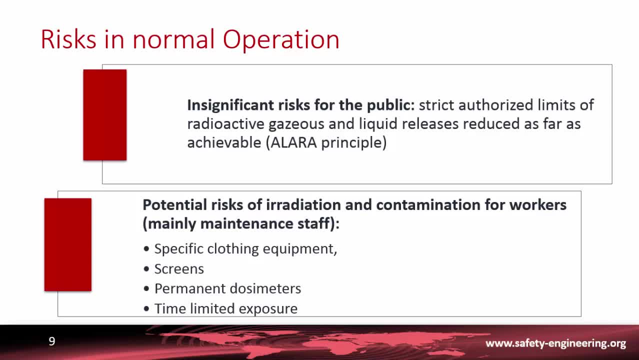 and the dose incurred is also permanently measured through dosimeters. So it is also important to limit the time of exposure and, for instance, before making some control in the steam generator tubes, the maintenance staff, the persons who make this inspection, are trained to jump in the box of the steam generator in order to limit the time it takes to make the job. 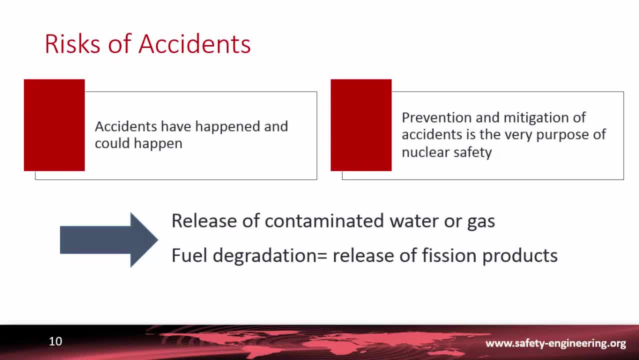 So the main risk is the risk of accidents, and accidents have happened and they could happen, And the prevention and mitigation of these accidents is the very purpose of nuclear safety, because the consequence of an accident is to release- potentially release- contaminated water or gas. 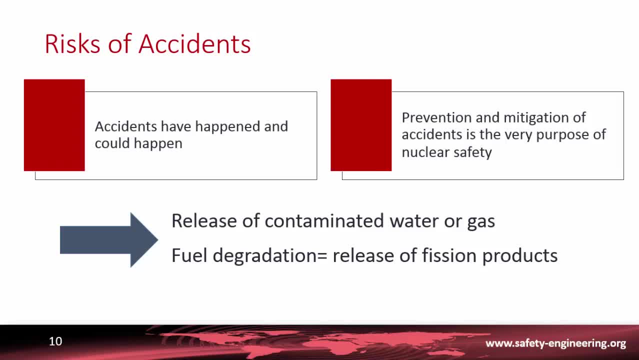 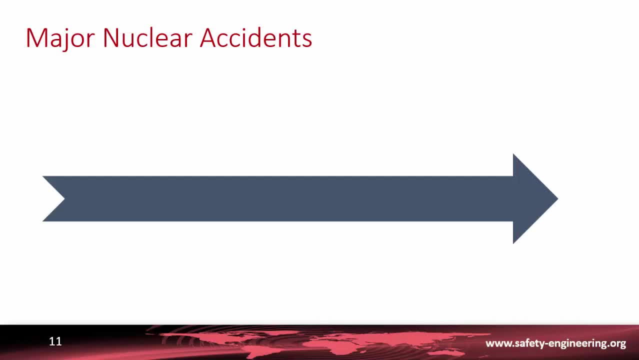 and if there is some fuel degradation there will be also the release of fission products. So we just mentioned here the three major nuclear accidents that have occurred in the world. The first one is the accident at Three Mile Island in the US in 1979..